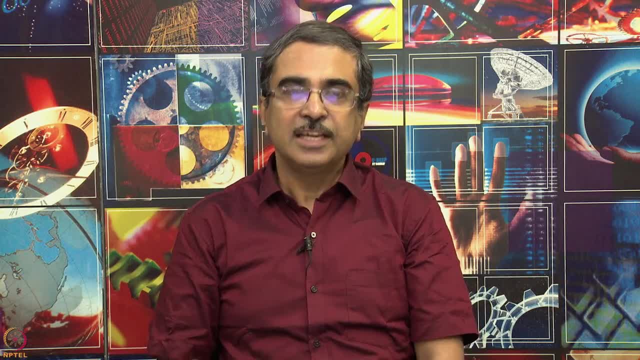 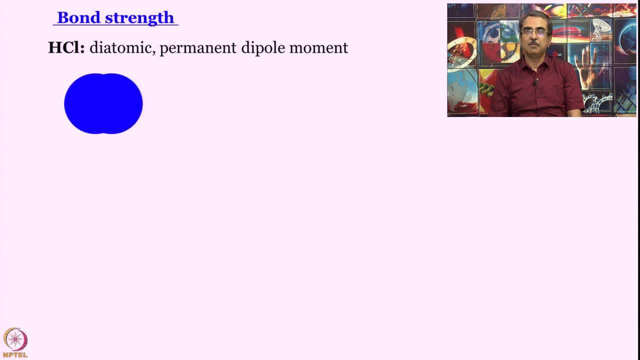 Here we are going to get an idea of bond strength. So again, let us work with the same molecule, say HCl. HCl is a diatomic molecule with a permanent dipole moment. So what happens when it vibrates? When it vibrates, essentially the dipole moment keeps. 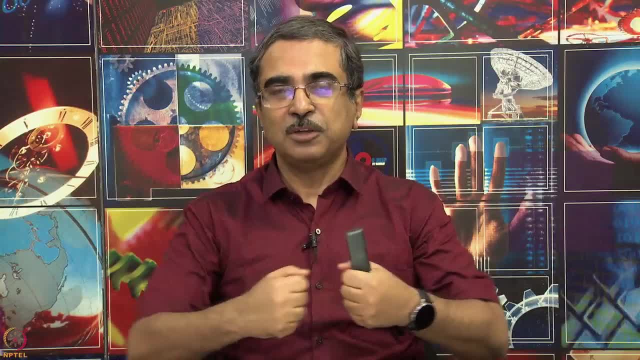 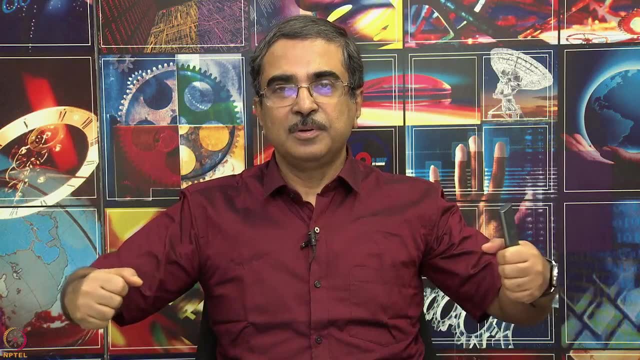 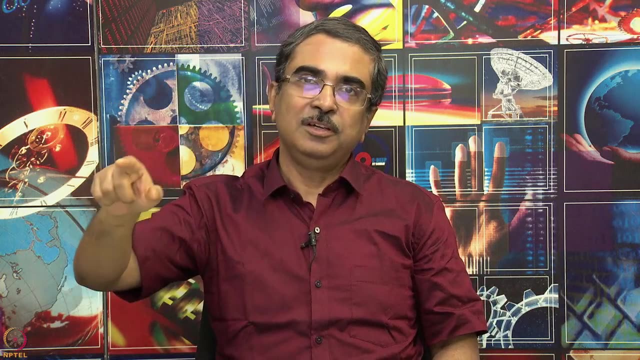 changing. So now you can think: if you now plot the dipole moment along this direction, what will happen? It will go up, then go down and then go up again. So again you get an oscillation kind of behavior, oscillatory behavior, But the graph will look a little different from. 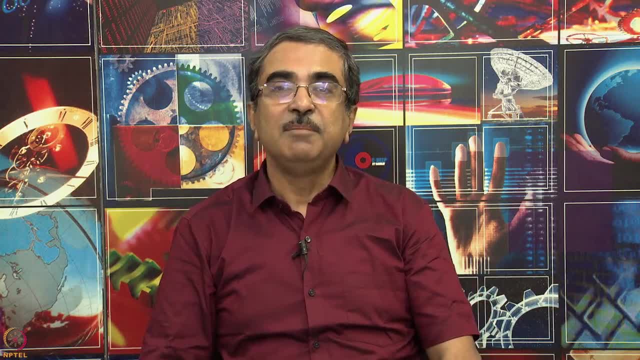 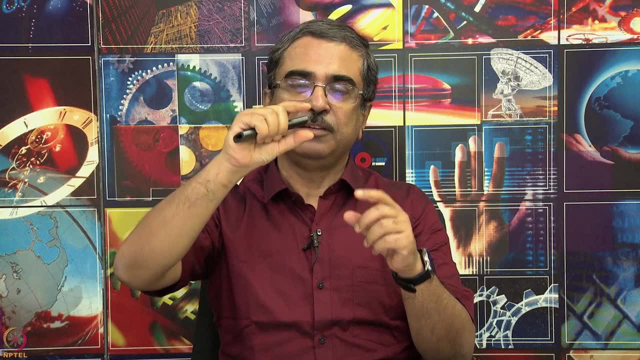 what it did earlier, because there is not going to be any minus sign, Because dipole moment will always point in one direction: It will be large dipole moment. well, something like this: keep on increasing, become large, then keep on decreasing to that value, keep on increasing. 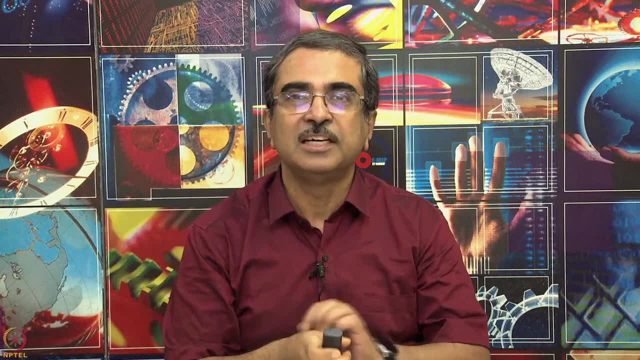 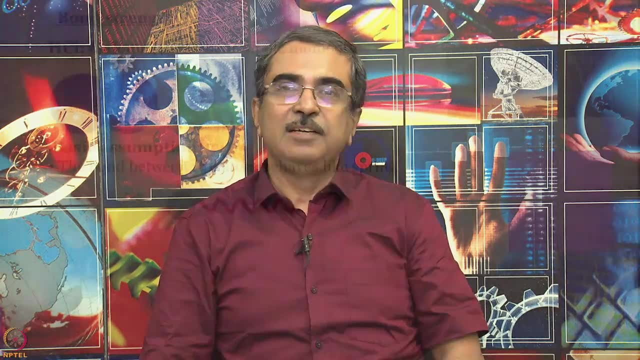 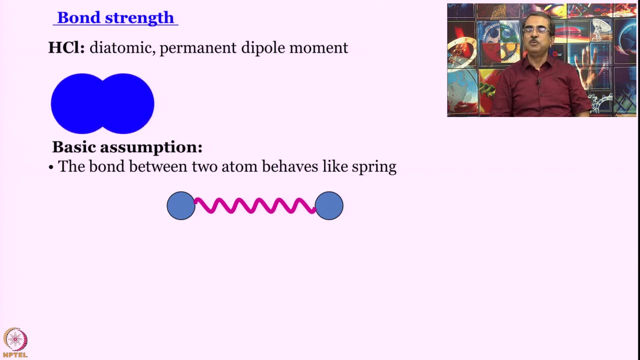 that. So that kind of a variation, So maybe sin square theta kind of sin square x kind of variation will be there. So the basic assumption in formulating the quantum mechanical treatment of HCl, to start with at least, is that the bond between two atoms behaves like a spring. 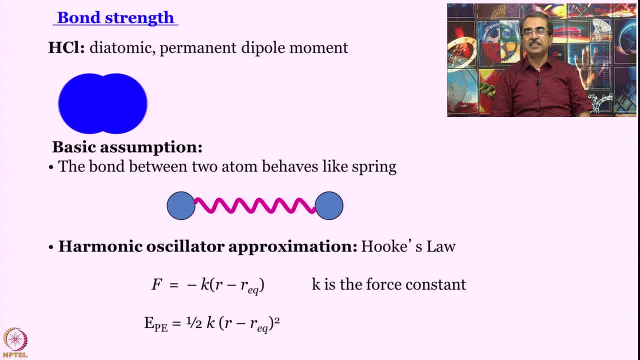 and not just any spring, a spring that is well behaved, a spring that follows Hooke's law. Hooke's law, you must have studied, is such where the force- restoring force- is proportional to the displacement And it is always towards the center. that is why you get this minus sign. 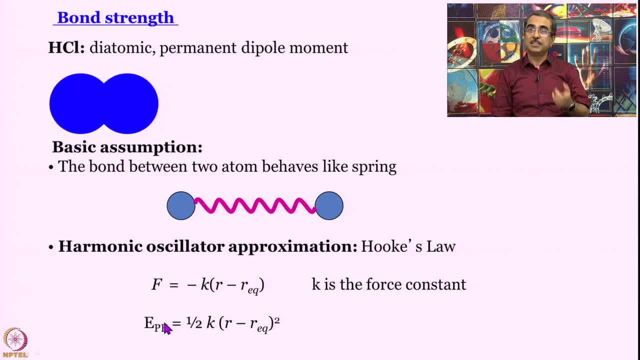 And potential energy. that comes here now for the first time we are encountering potential energy after hydrogen atom. For hydrogen atom molecule we did have potential energy, But here in rotations there was no potential energy. For vibrations potential energy is there And that potential energy is a parabolic potential half into k into r minus r eq. r eq is: 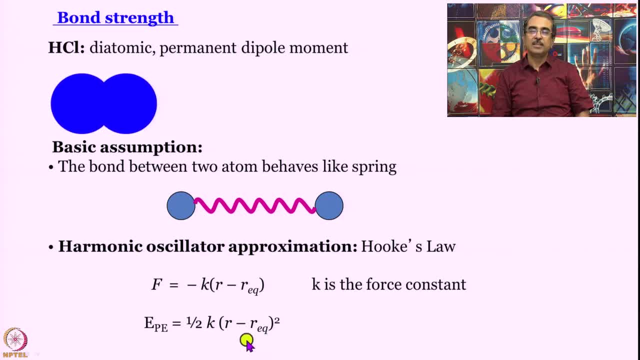 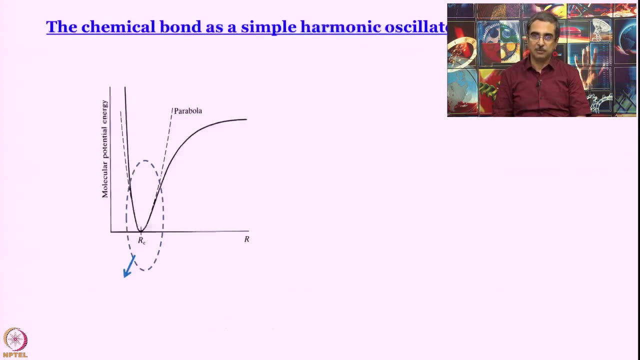 the equilibrium distance or equilibrium bond length. So deviation from that and square of that, that gives you the parabolic potential associated with harmonic oscillators. So harmonic oscillator is the approximation we are going to use, at least to start with. The question is: this is a valid approximation To answer that. we have plotted this. I hope you. 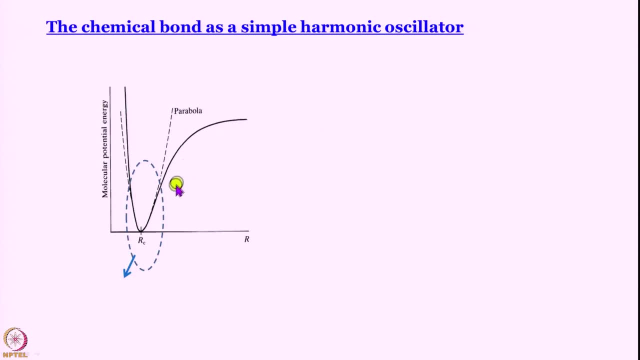 are familiar with this shape. now, This is what we obtained when we talked about, say, dihydrogen molecule. When two atoms very far away from each other, energy of interaction is negligible, Then they come close, close, close. energy keeps on increasing and decreasing Stability keeps on. 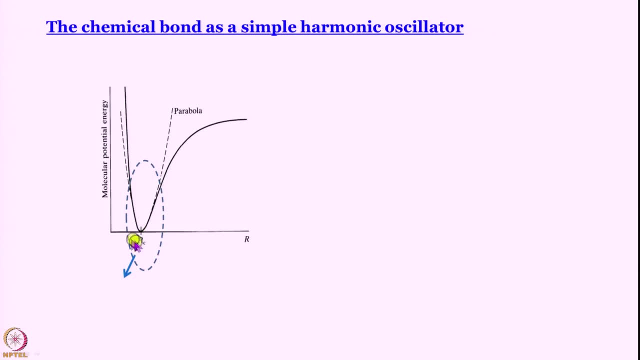 increasing goes to a minimum value at equilibrium bond length And then, for further approach, there is a sharp increase in potential energy. So this really is the potential energy surface, which is approximately can be modeled by something called a Morse potential, And this is definitely not. 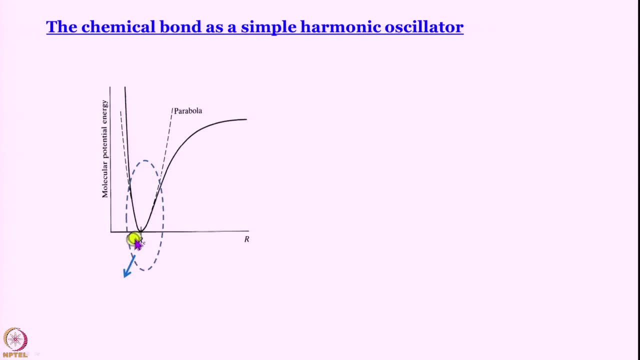 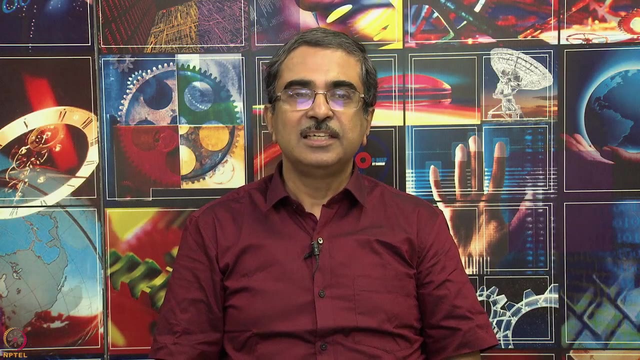 parabolic, But if I draw a parabola on it you can see that in this region for small displacement the parabola more or less holds up to here. then there is a deviation. Here also, then there is a deviation. So if you are content working with small vibrational energies, small displacements, 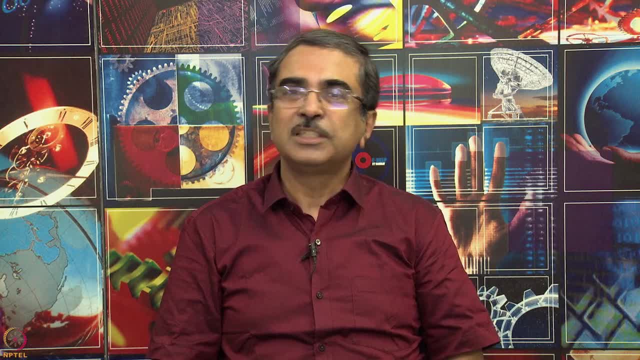 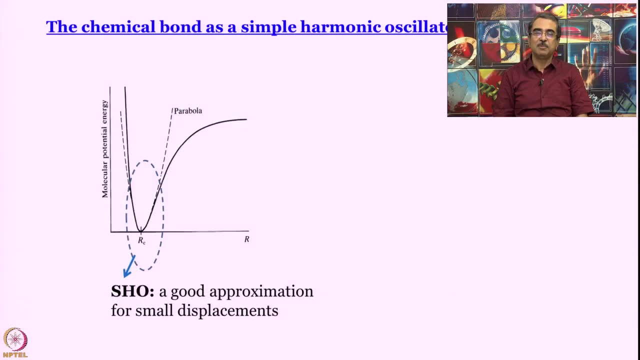 then the parabolic potential might work. We are starting with that kind of a hope. So we are starting with the hope that good, it is a good approximation, simple amount of harmonic oscillator for small displacements. So this is our parabolic potential and we 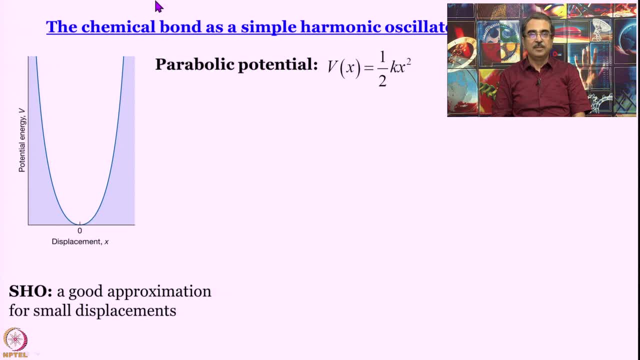 can plot it like this. Now we will write Schrodinger equation as usual. what is it? It is minus h cross square by 2 mu del square, plus half k x square. Remember once again we are using mu because it is a. 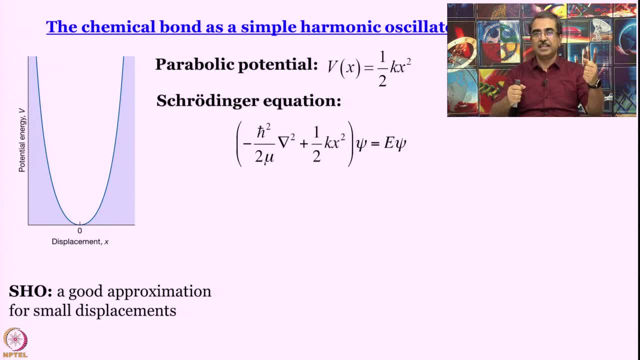 two body problem: h, c l. this is h, this is c? l. but we do not like two body problems more difficult to handle, So we reduce it to a one body problem, and when we do that, the mass that we need to consider is neither the mass of h nor the mass of c l, but rather 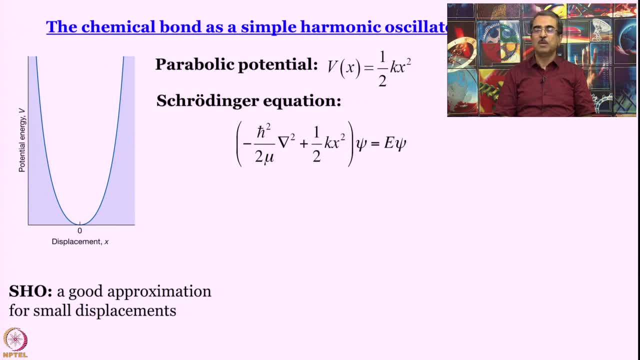 the mass, the reduced mass, 1 by mu equal to 1 by m 1 plus 1 by m 2.. So minus h cross square by 2 mu del square, that gives you the potential energy. half k x square, as we have discussed already, is the potential energy. minus h cross square by 2 mu del square gives. 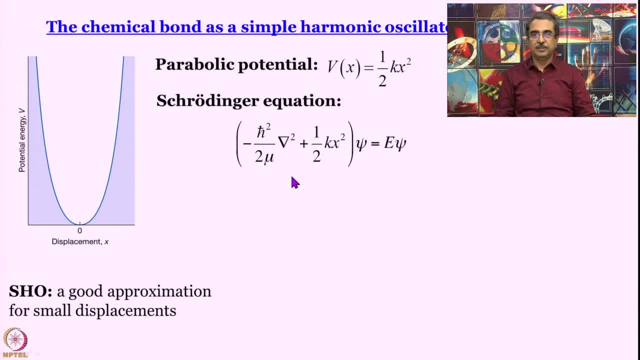 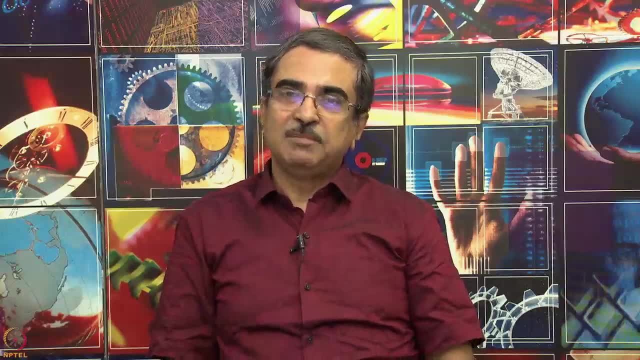 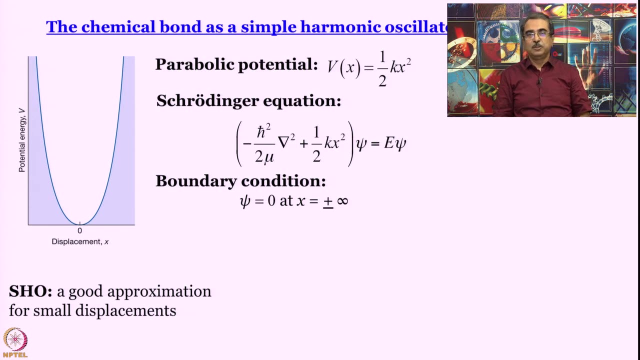 you the kinetic energy term of the Hamiltonian. So the Hamiltonian is there, we have written the equation, one can solve it. So the boundary condition that we have to use here- remember it is boundary condition that produces your quantization. So the boundary condition that we have to use here is psi equal to 0 at x. 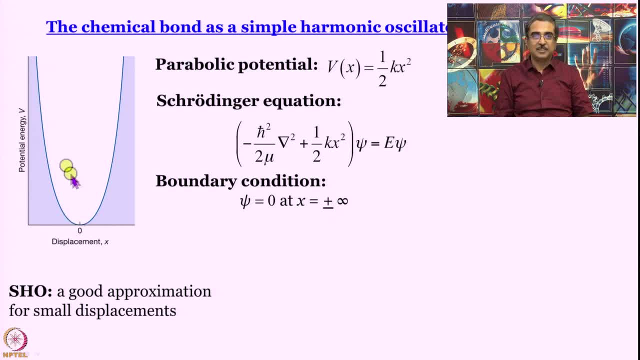 equal to plus, minus infinity. not at this surface, not at this surface. What is this surface? We have just plotted this parabolic potential For this value of x. what is the value of v? There is no reason to think that at this. 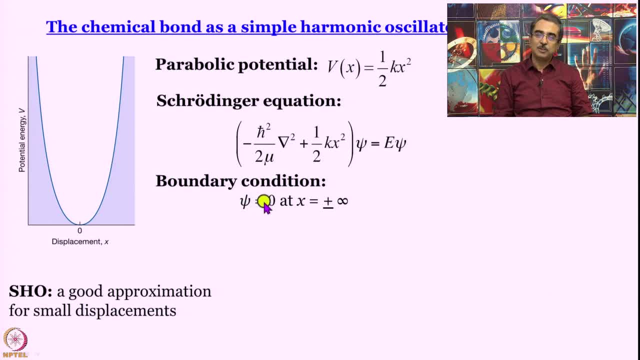 point, the wave function will become 0. It actually becomes 0 at x, equal to plus minus infinity. So, using that boundary condition, what you get is, first of all, you get quantization, you get different energy levels and you get this kind of wave function. Do they look like? 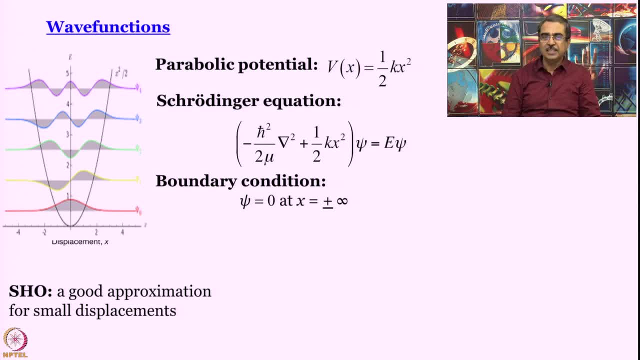 particle in a box wave functions- Partially, yes, they do look like sine waves- and even particle wave function- particle in a box wave function. you had no node for the lowest energy. one node in the next, one, two in the next, and so on and so forth. But these are 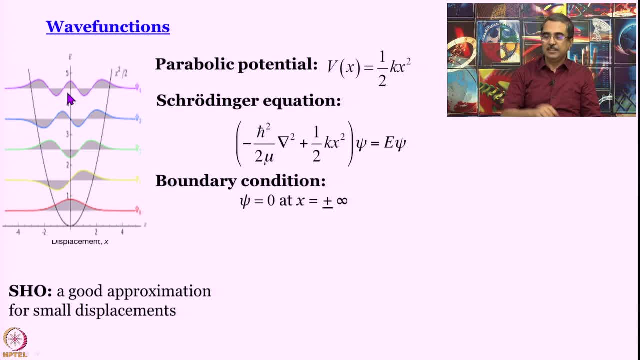 not really sine waves, So these are something like this. let me just write it here. So this is the wave function, Okay, Okay, So psi v is equal to normalization, constant n v multiplied by e to the power minus. for. 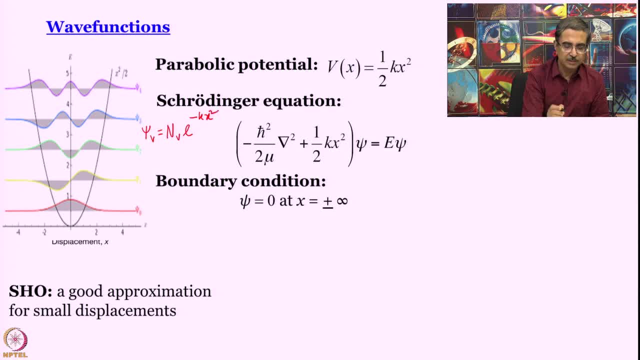 now I will just write k, and here I will just write k x square, since we are just trying to give you an idea. this is a Gaussian function And this is multiplied by what is called a Hermite polynomial in x. What is a Hermite polynomial? Please refer to our lecture series. 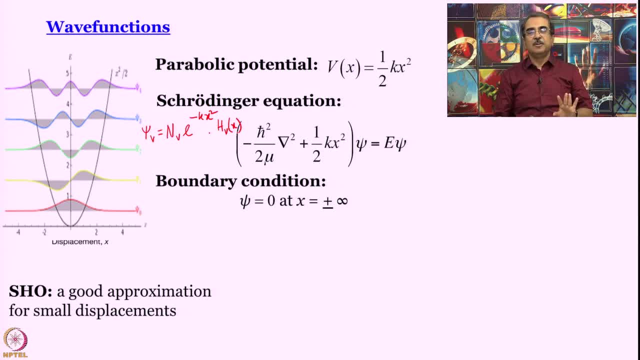 We are not going to delve further here. Unfortunately we will not go into that, So let us just try to do a little bit of a analysis. Unfortunately, in this course, you will have to believe me when I say that this is a form. 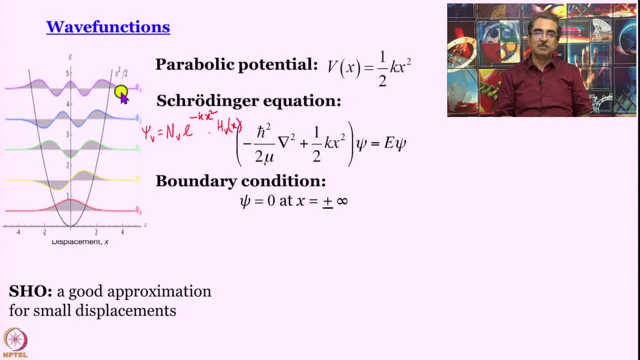 And when you plot this, this kind of a function is obtained. it becomes 0 only at plus minus infinity. So you can see some wave function outside the area, that where we have drawn the potential energy surface also. Okay, This is the quantum mechanical description of simple. 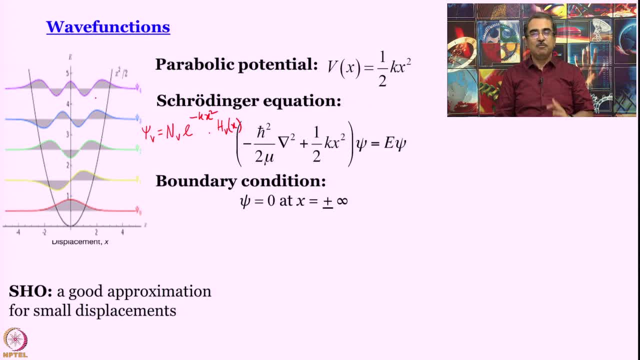 harmonic oscillator. Quantization is there. Wave functions are there. So the wave functions are here, So the wave functions are there. So what is the quantum mechanical description? So the only thing that remains to be told at this point is: what are? what is the expression? 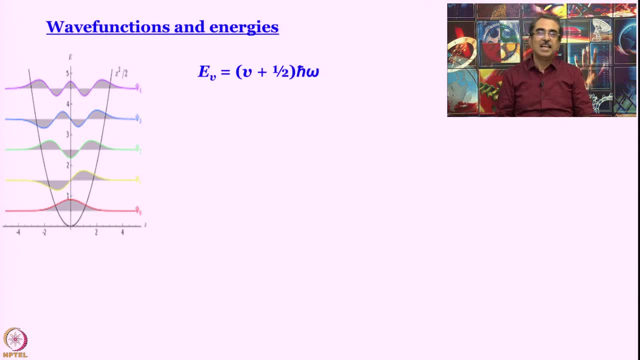 for the energies. This is the expression for energies: ev equal to v plus half, h cross, omega. h cross, you know, h by 2 pi. omega is the angular frequency of vibration. v is the vibrational quantum number goes from 0,, 1,, 2, 3, so on and so forth. 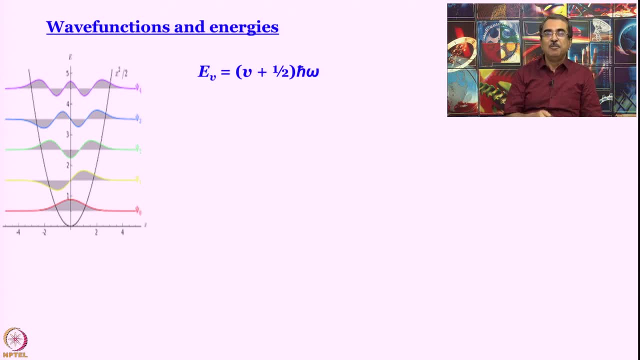 Now we have an interesting situation. if you put v equal to 0,, what is ev going to be? It will not be 0, it is going to be half h cross omega. So this energy is called 0 point energy. what it essentially says is: if it was a classical, 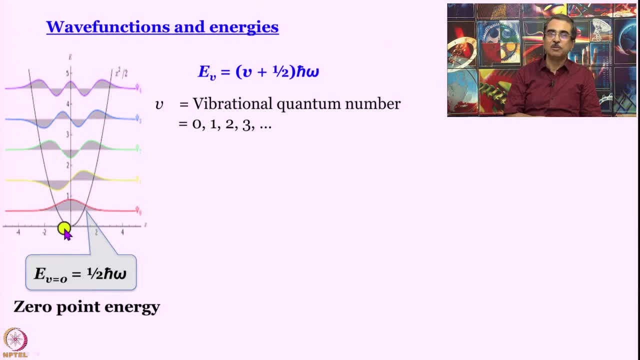 simple harmonic oscillator. it could have gone down here to the bottom of the well and it could have had no energy at all, which means it would not vibrate. However, for a quantum harmonic oscillator it is not possible to have 0 energy. 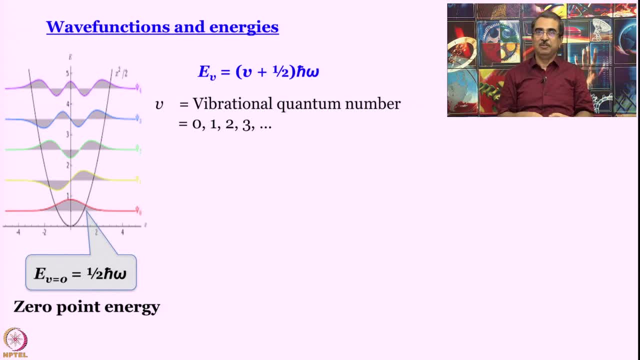 The oscillator is going to oscillate even at 0 Kelvin. that is why it is called 0 point energy. Why is that so? That is so because otherwise, you know, uncertainty principle will be violated. So we have a quantum harmonic oscillator. fine, so it is vibrating. 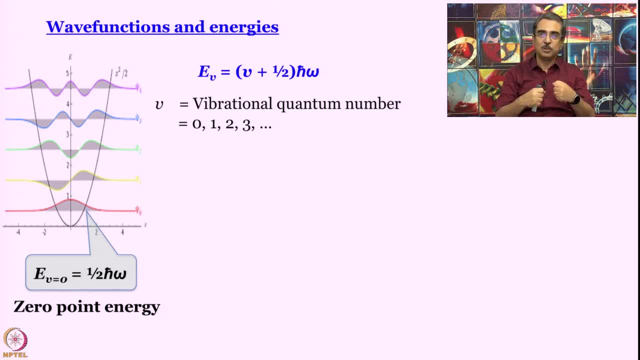 Let us say I keep on decreasing temperature and it stops. It drops to the lowest possible level. vibration energy goes down, down, down and then it stops. Now we know the separation r: 0, that means we know position, we know the momentum exactly. it is 0. So position and momentum are both determined accurately. that violates uncertainty principle. So in order to ensure that it does not violate uncertainty principle, poor quantum harmonic oscillator has to oscillate even at 0 Kelvin with 0 point energy. 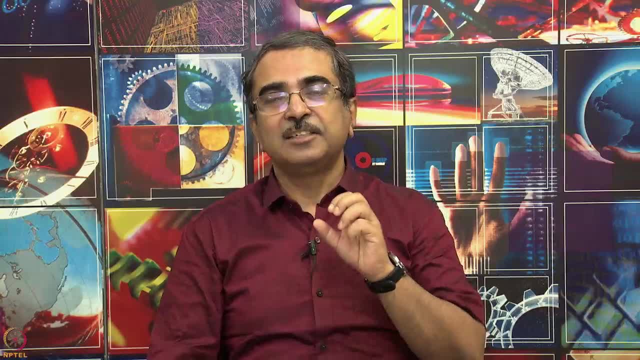 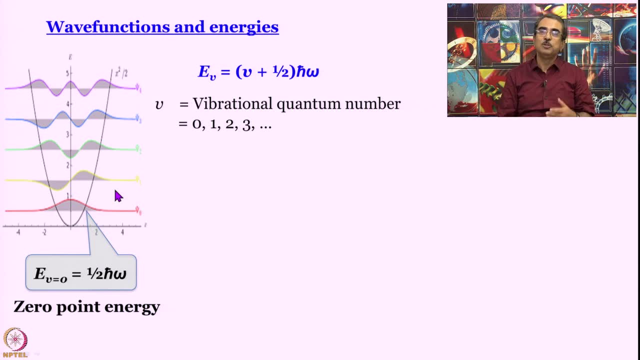 So we have a quantum harmonic oscillator With 0 point energy. in fact, at room temperature, only this level is populated because the separation is something like 1000 centimeter. inverse, If you use Boltzmann distribution you will find that population of this even your v equal. 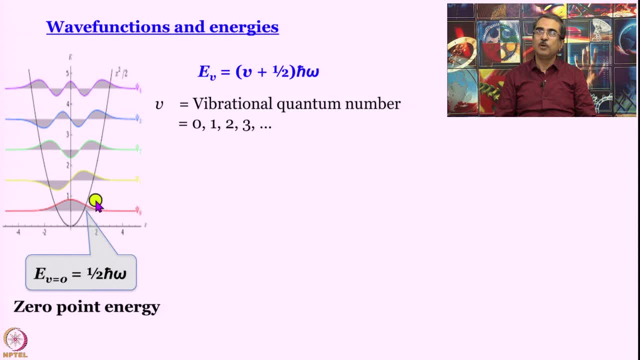 to 1 state is going to be 0.008 or something. only 8 will be in v equal to 1 state and it will fall off rapidly. So if the ratio is 1000 to 8, what will? the ratio 8 is to something b, it will be practically. 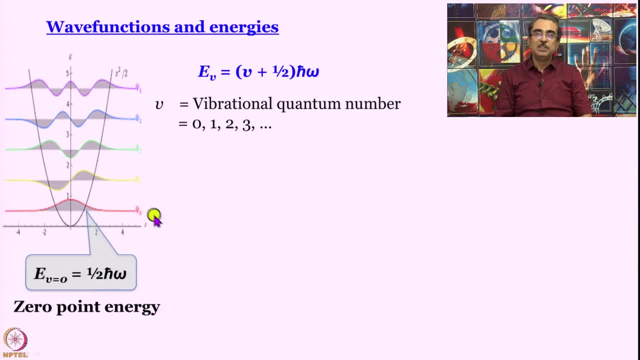 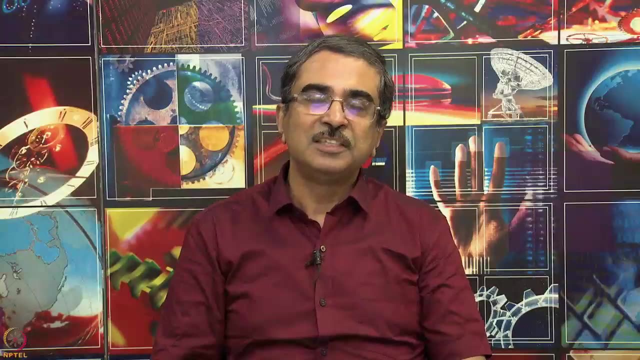 0. So only the v equal to 0 level is populated at ground state for all practical purposes. So all transitions actually originate from there. that is very important to understand. That being said, there is more interesting stuff coming up. 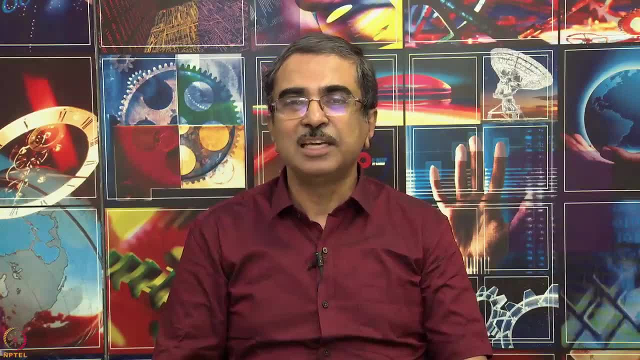 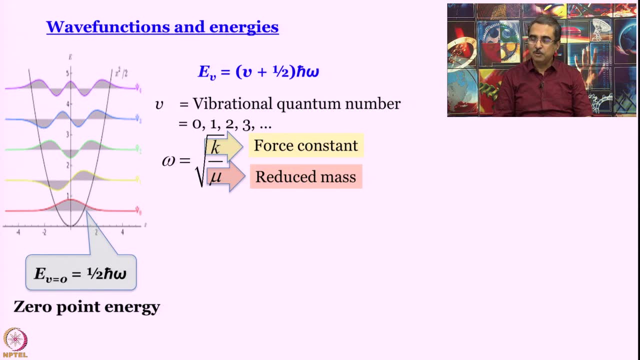 We know that angular frequency for a simple harmonic oscillator is root over k by mu. k is force constant and mu is reduced mass. So if we somehow determine omega, then we should be able to determine force constant, provided I know which atoms I am working with. if I know which atoms I am working with, I 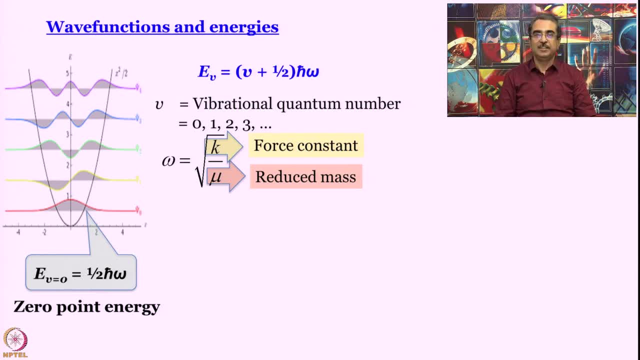 know their masses. How do I find this? let us see What is the energy gap between two successive levels: e v plus 1 minus e v. do the math very simply: write v plus 1. here v and v will cancel. 1 minus half is half, so you. 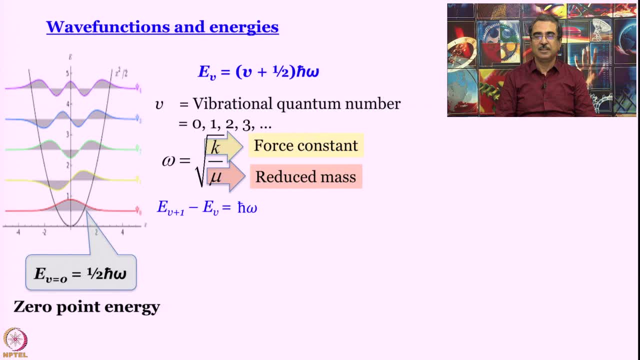 are left with h cross omega, So sorry, half will also cancel. since I made a mistake, I will write it: e v plus 1 is equal to v plus 1 plus half multiplied by h cross omega. so e v plus 1 minus e v. 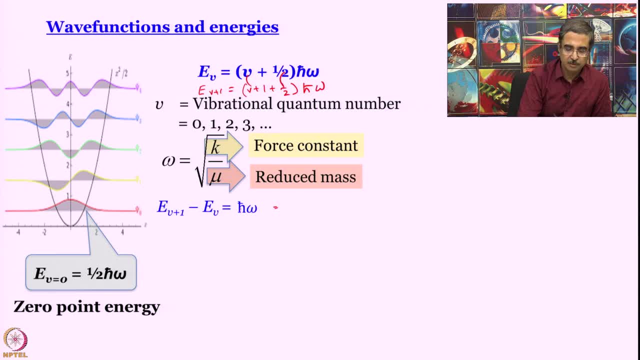 is equal to well, v and v. cancel half and half cancel, you are left with h cross omega. Now, what is this omega? remember, it is a angular frequency of vibration, and if you think why I am saying this again, you will see very soon. why angular frequency. 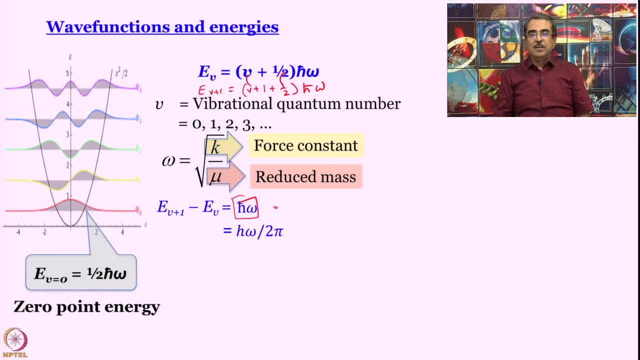 of vibration. So instead of writing h cross omega, I can write h omega by 2 pi. fair enough, what is omega by 2 pi? omega by 2 pi is nu, so this becomes e v plus 1 minus e v is equal to h. 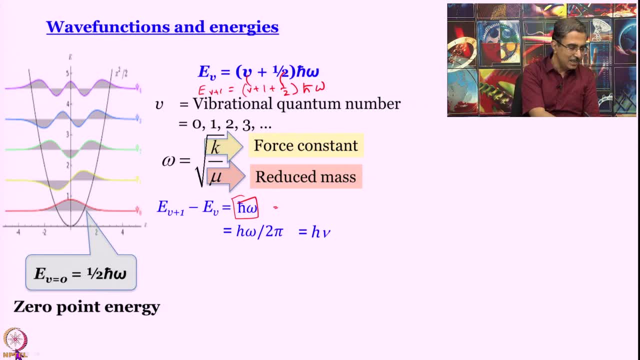 nu is nu. Nu is the frequency of vibration. I might as well write like this, But now we are in an interesting situation. What is there on the left hand side? Ev plus 1 minus Ev, that is delta E. Do you remember what delta E is? We have written that it is called Bohr. 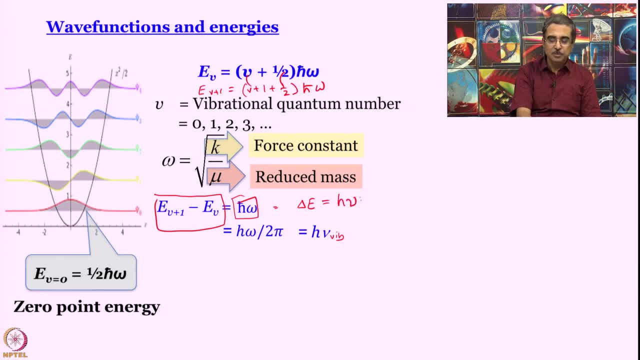 resonance condition that is equal to h nu light. So what it turns out is that this h nu light is equal to h nu vibration. h and h cancel you are left with. nu light is equal to nu vibration. So a simple harmonic oscillator would absorb only that light. Well, for delta V equal to one. 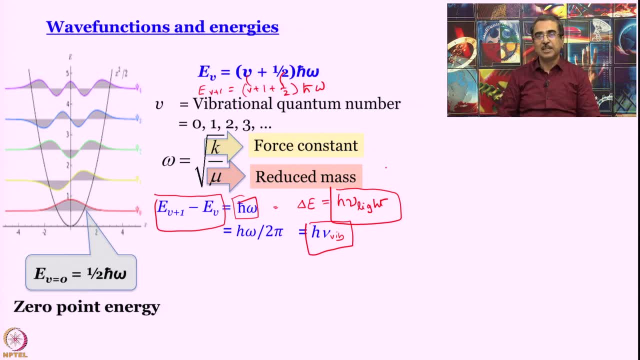 kind of transition, which is the only transition that is allowed. it is going to absorb that light which whose frequency is exactly equal to the vibrational frequency. That is something that I find to be very amazing. So you can write like this: vibrational frequency. 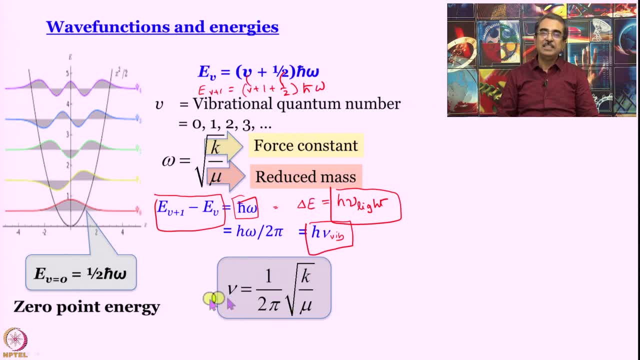 is 1 by 2 pi root over k by nu. we know that. So that is equal to frequency of light as well, And it is conventional in vibrational spectroscopy, like in rotational spectroscopy, to work with not frequency but wave number. So nu bar becomes 1 by 2 pi c multiplied by root of. 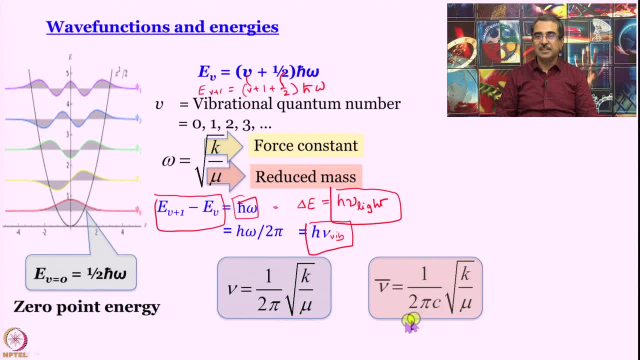 k by mu. So this here is an expression of light that would be absorbed for a V to V plus 1 transition, and that has k in the numerator, mu in the denominator. If you know mu, you can easily find the force constant k. What would the force constant k tell us about? It tells us about how. 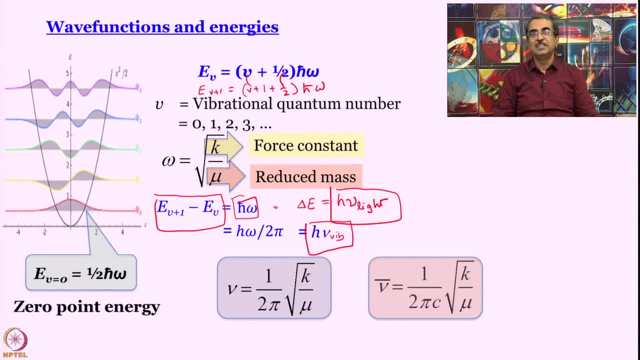 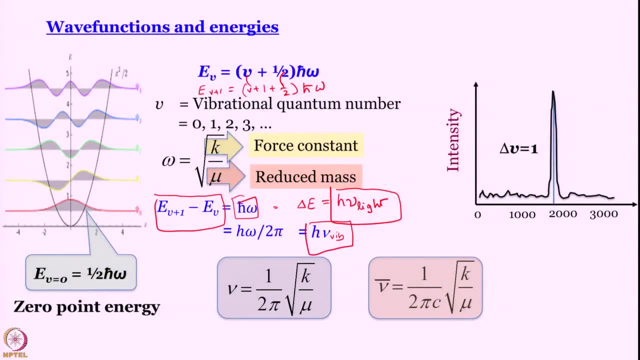 strong the bond is, so it can determine bond strength. What would the spectrum look like? Actually, it would look like this: this one single line. of course, there would be some width and all. but for delta v equal to 1, even if the transitions originated earlier, it does not matter, it will always be just h, new wave. 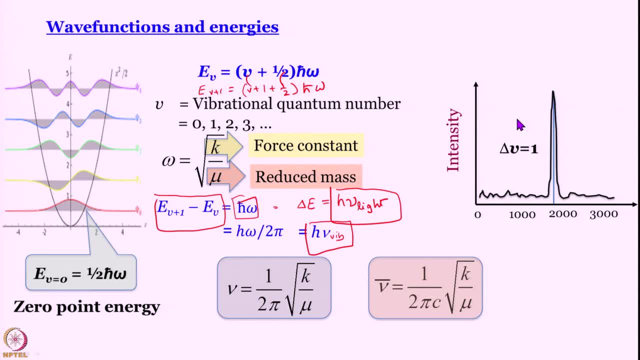 So a single line is expected in the spectrum of simple harmonic oscillator. more so because, in any case, all transitions begin from v equal to 0 at room temperature. The selection rule is delta v equal to 1. how do we get it? please refer to our spectroscopy lectures. As usual, we will not close. 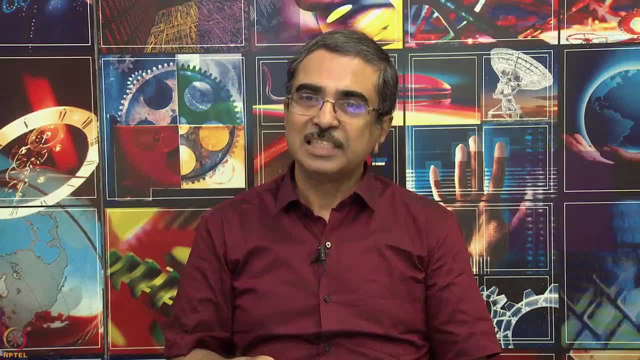 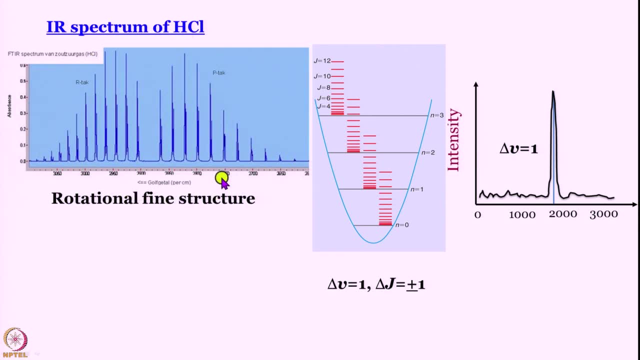 the discussion without showing you an actual spectrum. this is the expectation. one single line. this is the reality. if you use a good enough IR spectrometer, a high resolution IR spectrometer, instead of one band, you get, well, two branches of lines. where do these branches arise from? 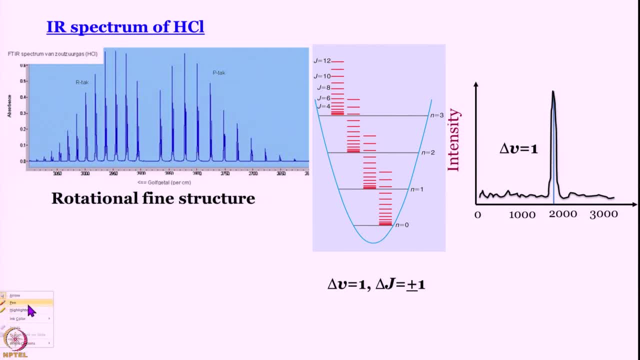 These branches arise from the fact that every vibrational level is associated with rotational levels. now you might remember here that we said that rotational levels are such that the higher levels are populated. why are they populated? because the energy gap is so small. higher vibrational levels are not. 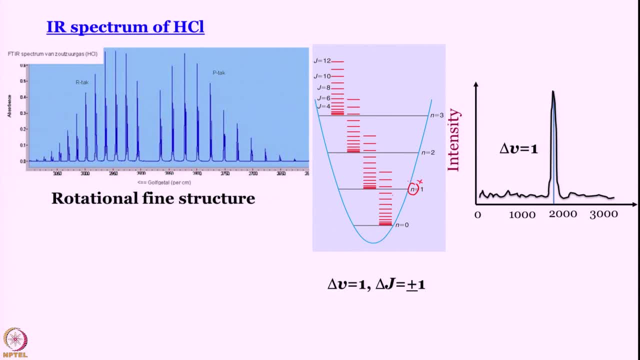 populated. here we have written n. this is not populated much because the energy gap is too large, but for n equal to 0. So all these levels will be populated in the same ratio as is predicted by Boltzmann distribution. So now upward transitions can actually begin from any of these levels. 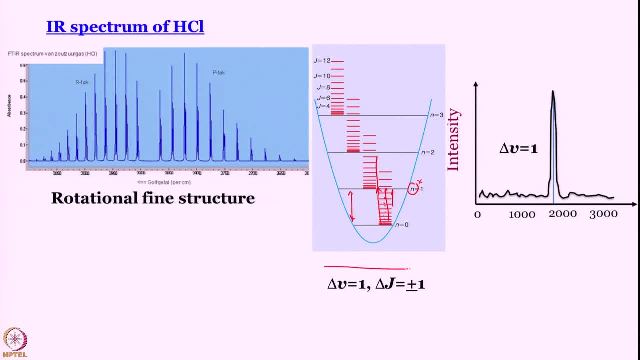 So you get arrows of different length and, without going into further detail, let us just believe this again: that the selection rules are delta v equal to 1 and delta j equal to plus 1.. So you get arrows of different length and, without going into further detail, let us just believe this again: that the selection rules are delta v equal to 1 and delta j equal to plus 1.. 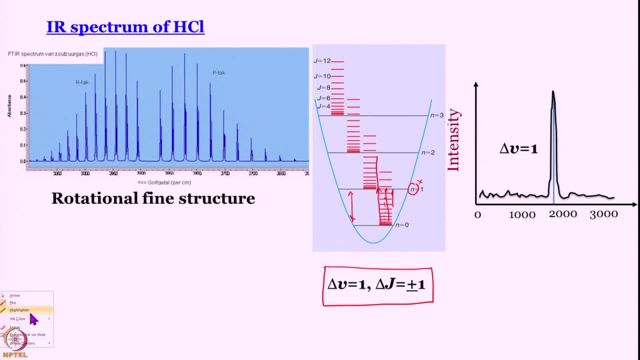 So you get arrows of different length. and without going into further detail, let us just believe this again, that the selection rules are delta v equal to plus 1 and delta j equal to plus 1.. Meaning, if you start from a j value, let us say I cannot make out which j it is. let us say it is j equal to something 3.. So from here, 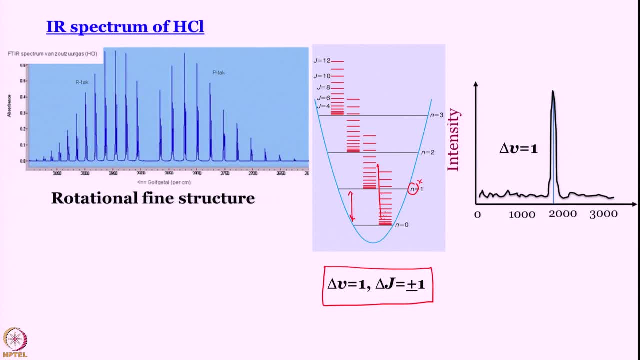 you will be able to go to only particular j values associated with the v equal to 1 level. Now I recommend that you work out the expression of energies associated with this kind of transition from Banwell and McCash's book. I am not doing it here because it is very, very simple: algebra. 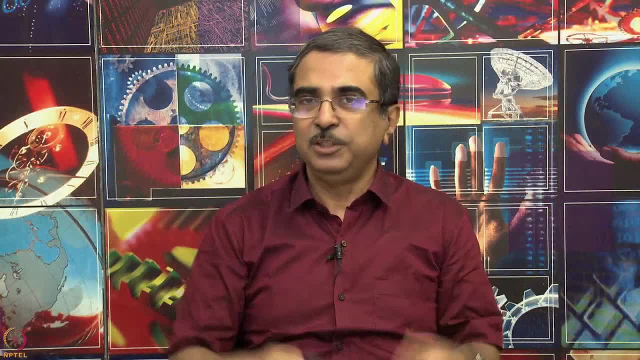 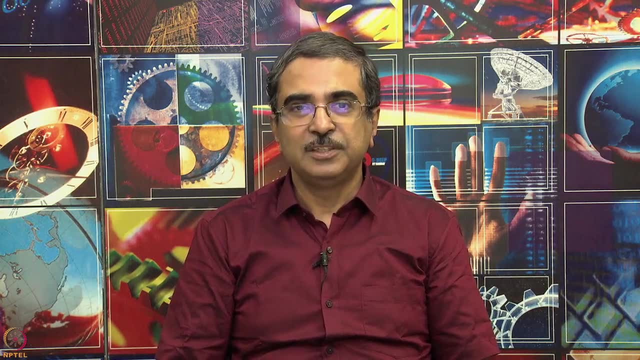 for those who are going to take this as an NPTEL course. if you want, we can do it in the interactive session. others: if there is any problem, please write me an email or something and we will do it. So we get two lines. these are called the p branch and the r branch. as you might notice that there is 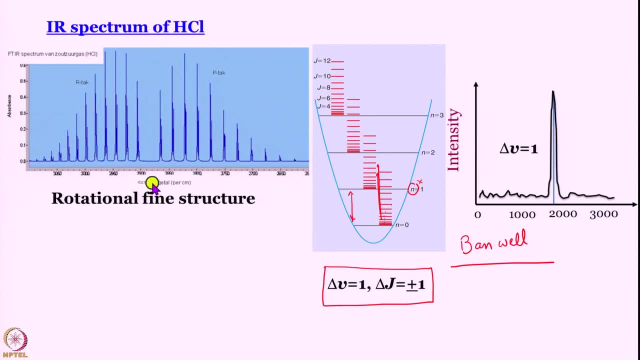 nothing at this point. So you get two lines. these are called the p branch and the r branch. As you might notice that there is nothing at this at the center, where the line was expected to be. that is because you have delta v equal to 1. 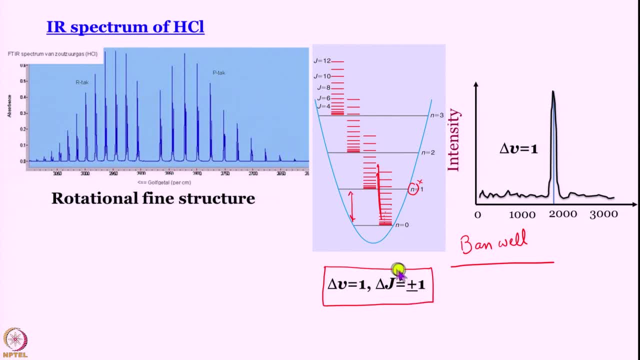 delta j equal to plus minus 1 delta j equal to 0 is not there. that is why you get this kind of an expression and this kind of a line. So from one spectrum, if your spectrometer is good enough, you can get an idea of ir, which gives you an idea of bond strength, as well as you can get an idea of 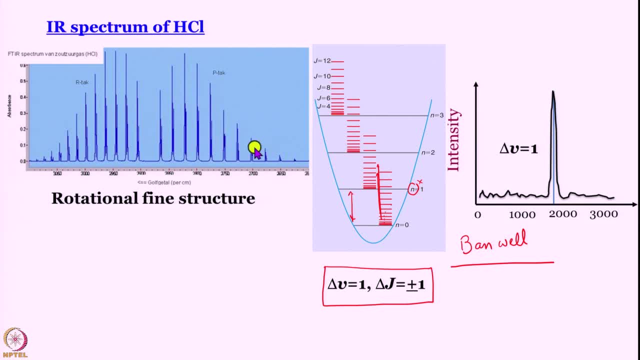 separation of rotational levels. the separation is going to be 2B once again, So you can get an idea of bond length and bond strength from the same experiment if your IR spectrometer has high enough resolution. This one more thing: if you zoom into one of these lines, unfortunately it is flipped here. 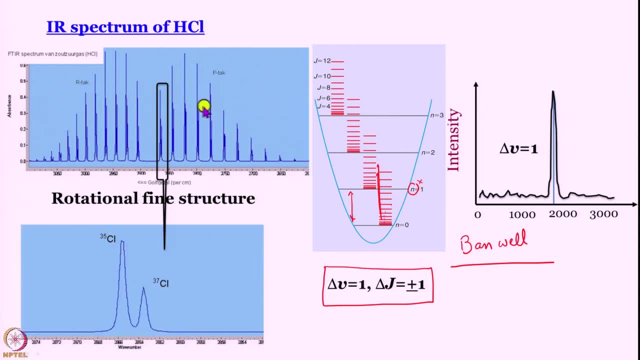 for whatever reason, you see that each line is actually a doublet. there are two lines associated with it. Why Go back to class 8 level chemistry? remember? chlorine occurs in nature as two isotopes: chlorine 35 and chlorine 37, atomic weight of 35.5 is just an average. So when you do the experiment, 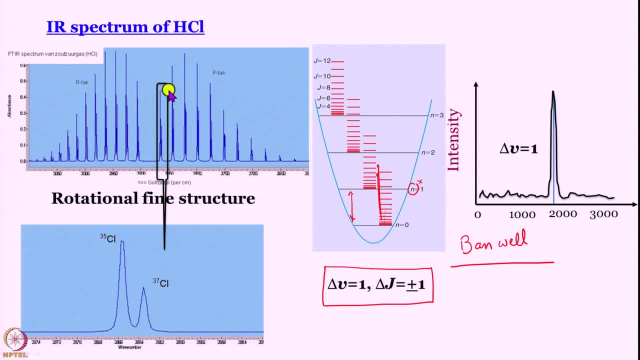 you actually sample individual molecules, So they are either HCl with chlorine 35 or HCl with chlorine 37, and here you get two different lines from for chlorine 37 and chlorine 35. The isotope effect shows up very, very nice. 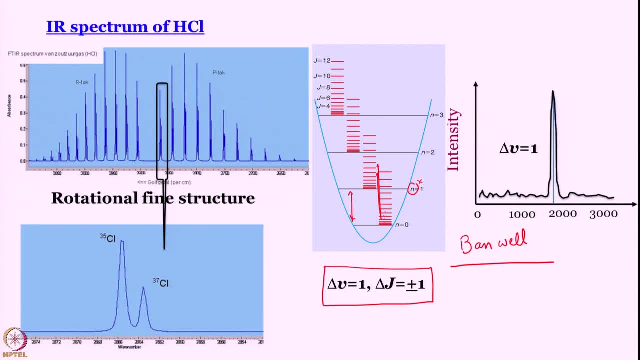 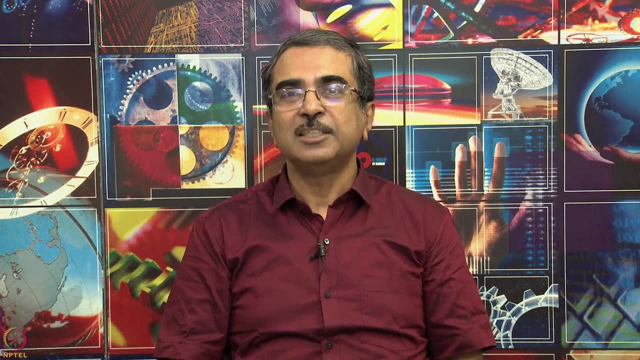 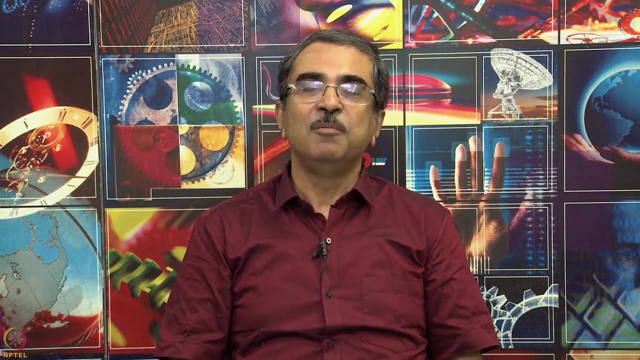 In this high resolution what is called row vibrational spectrum as well. So we get an idea of isotope abundance, isotope abundance, relative abundance of isotope. We get an idea of relative abundance of isotopes as well from high resolution IR spectra. 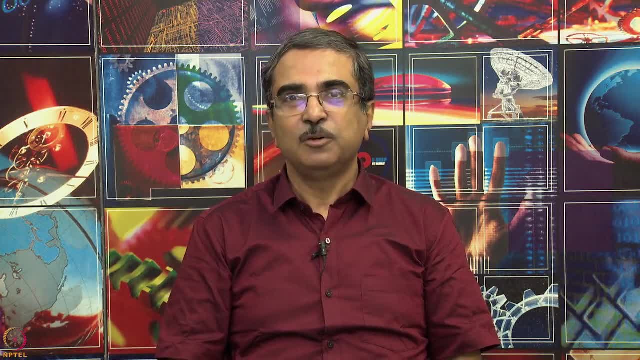 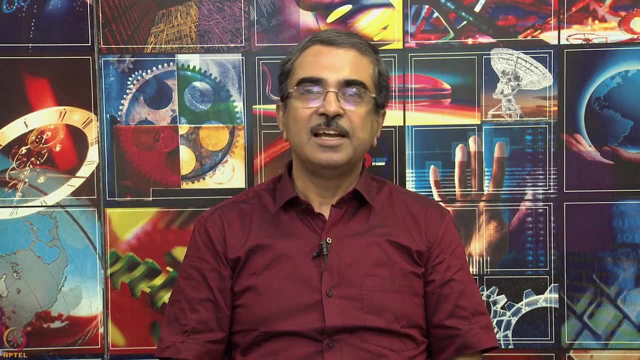 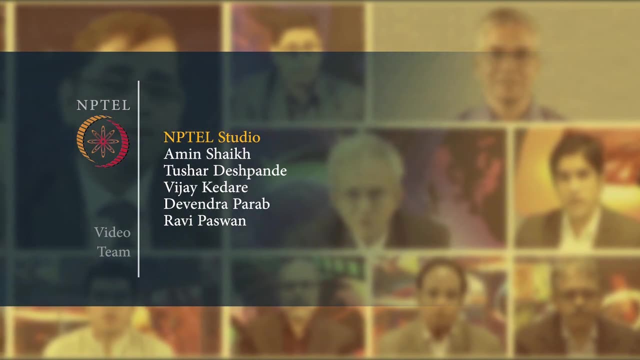 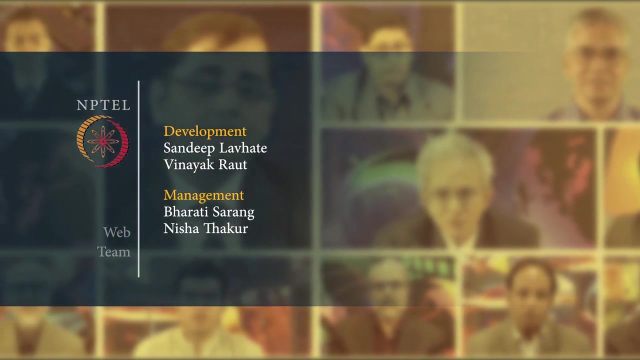 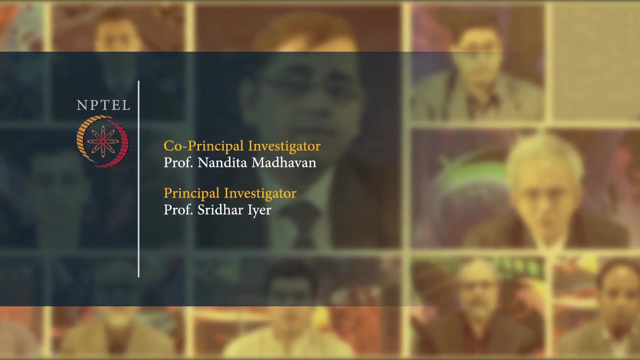 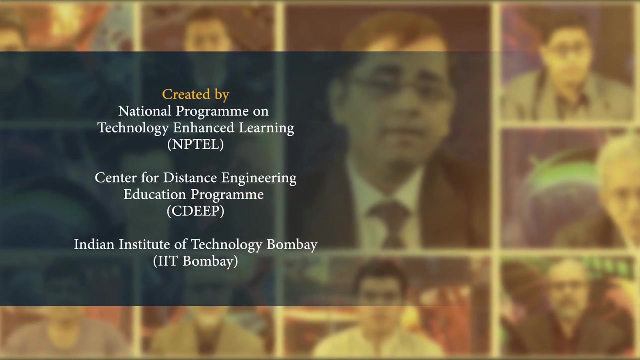 which are often called row vibrational spectrum, rotation vibration. So row vibrational spectrum. So much for vibration and rotation. Next we are going to go into electronic spectroscopy. So we are going to go into electronic spectroscopy and we are going to look at how to do that.